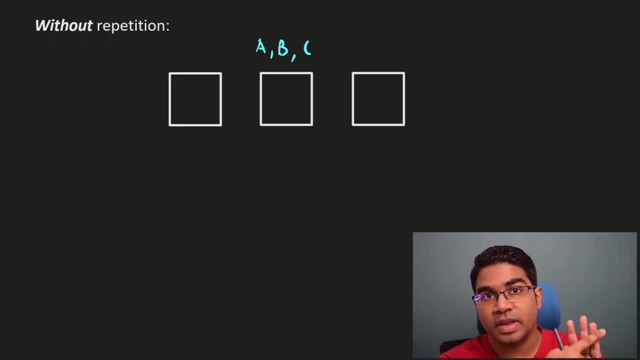 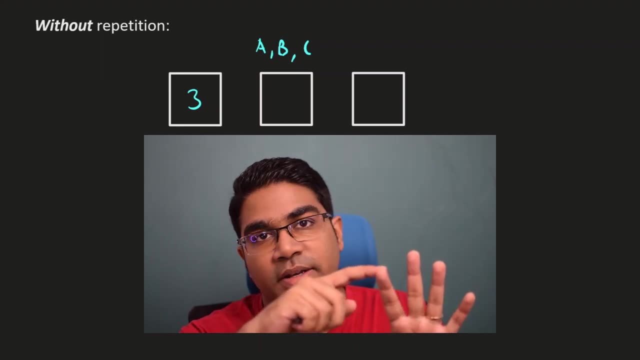 So for the first position we still have all our choices because we haven't used any of them. So we have three for the first position. Now, in the second position we've already used one of the letters. So out of the three we've already used either A, B or C. 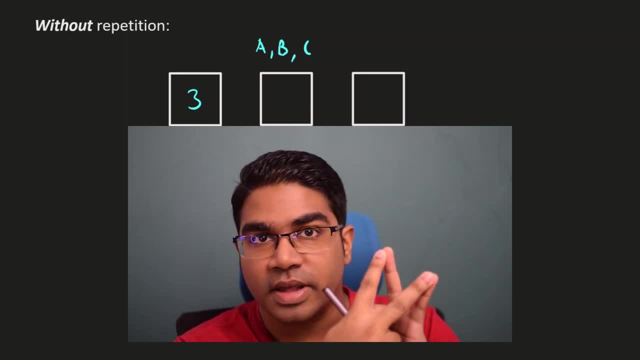 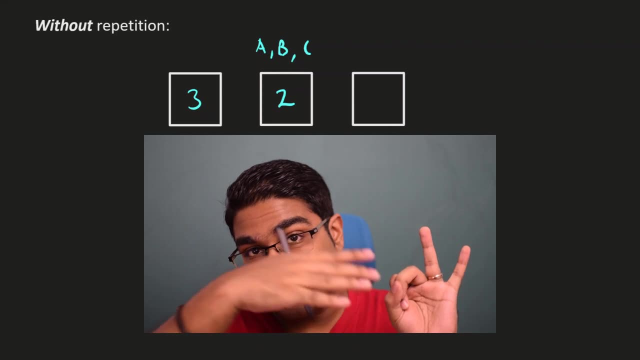 Whichever one we used now, we only have two choices left. So in the second place we can only arrange two different letters, And for the third place, the third position, we've already used two letters, Two of the letters, Two out of three of the letters. 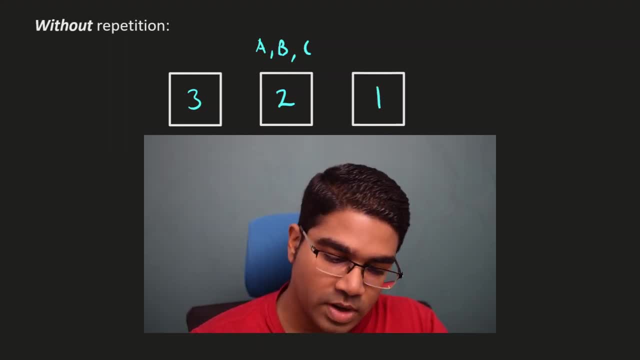 So we're only left with one. So we can only arrange one in the third position, Using the multiplication rule again, the total number of ways will be three times two times one. This will be six ways. So what we've done here actually is a permutation. 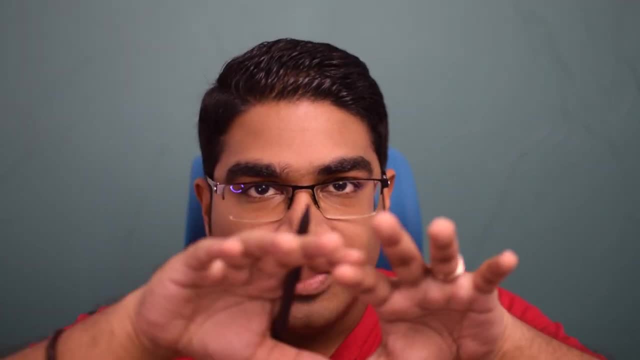 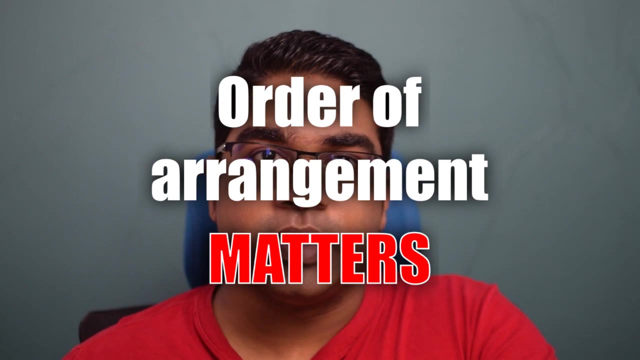 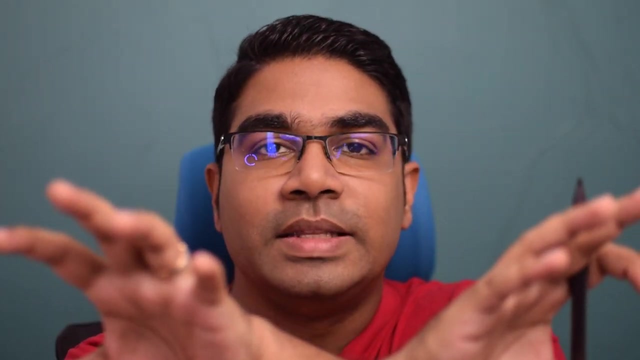 Permutations are numbers of ways to arrange something. The key word in permutation is arrangement. Arrangement matters, in permutation The position matters. If I have two and one and I switch them to be one and two, these are considered two different arrangements. 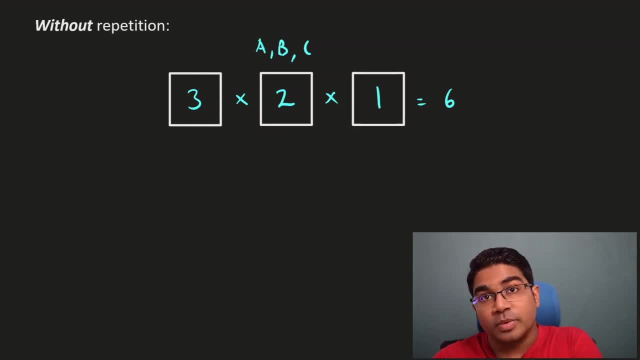 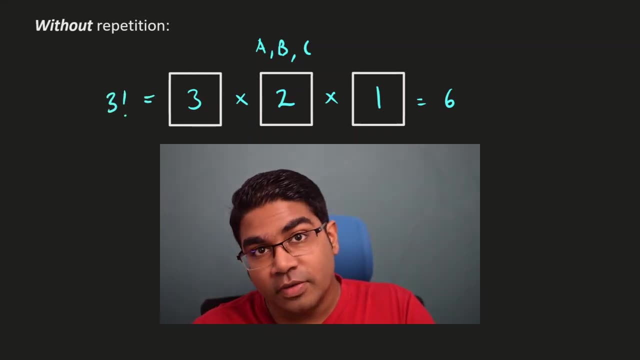 They are not the same thing. So this multiplication here three times, two times one can also be written as three factorial. So factorial means you take the number and multiply by the number before And the number before until you reach one. Let's use another example here. 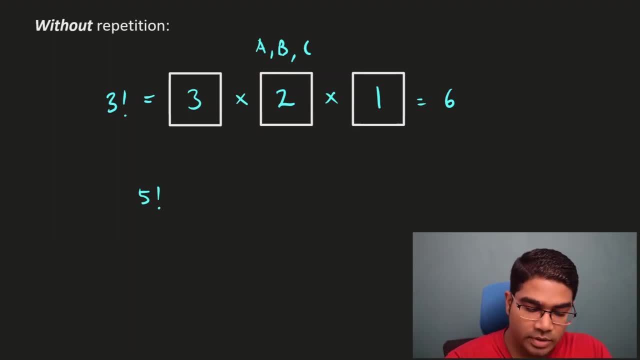 Let's say we have five factorial. Five factorial is actually five multiplied by take the number before, four, multiplied by do the same thing again three times two, until we go to times one. Then we stop. So this is known as factorial. 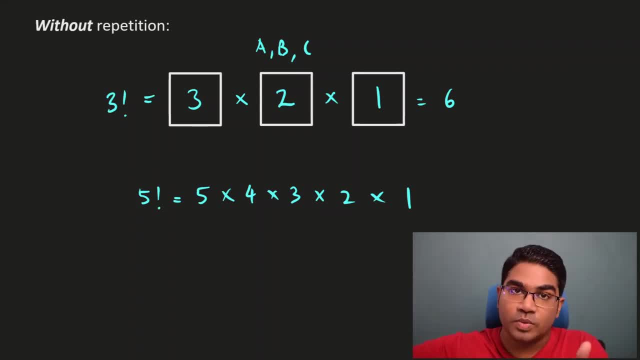 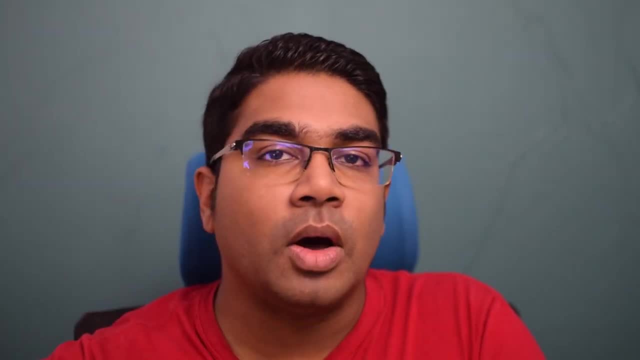 Five factorial, So it will be five times four until you get times one. We are going to keep using factorial in this topic, So it's very important that you understand what this is. Now let's do some operations using number factorials. Let's look at the first one. 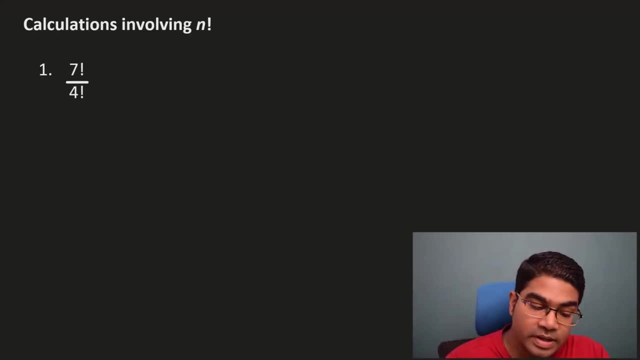 Seven factorial over four factorial. This can be written as seven times six until we get times one over four factorial. Now I'm going to leave four factorial as it is because I want to show you how we can eliminate it. Now, if you look carefully, 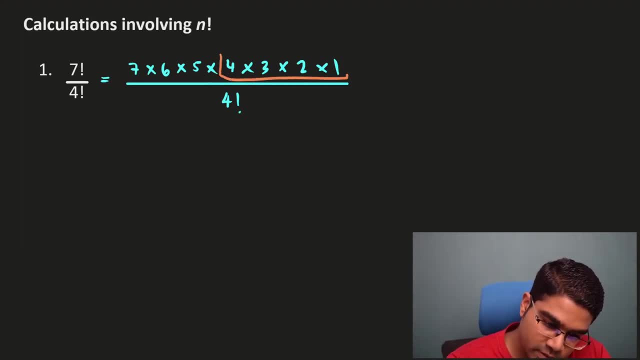 four times three times two times one, This is four factorial. So we can actually write this down as seven times six times five times four factorial. That means we do not write until times one divided by four factorial. So now we can actually divide four factorial and four factorial to get one. 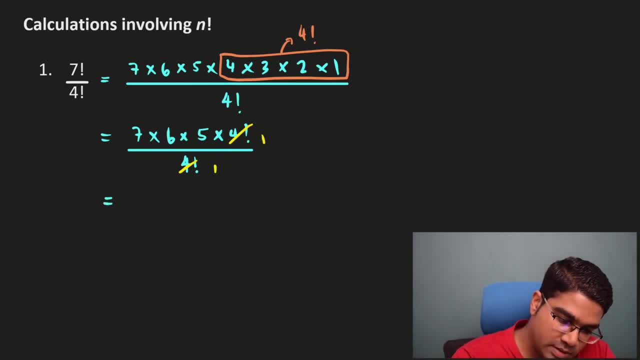 So this will simply become seven times six times one, Six times five, That is seven times thirty, which is two hundred and ten. Let's try another one: What is six factorial divided by three factorial times three factorial? So here we can write it as six times five times four. 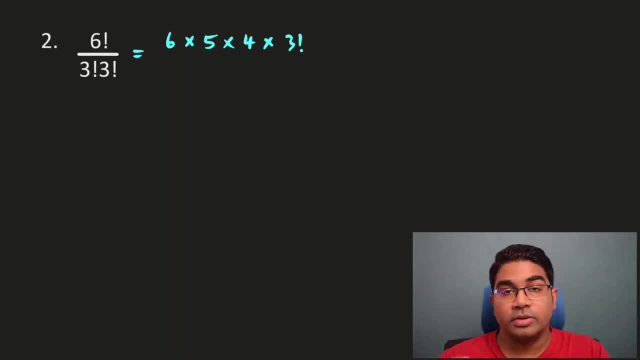 And we write three factorial here because we are going to divide by three factorial in the denominator, So we leave it at that, So this divided by three factorial times. We don't want to write the other three factorial as three factorial because there is nothing to cancel out at the numerator. 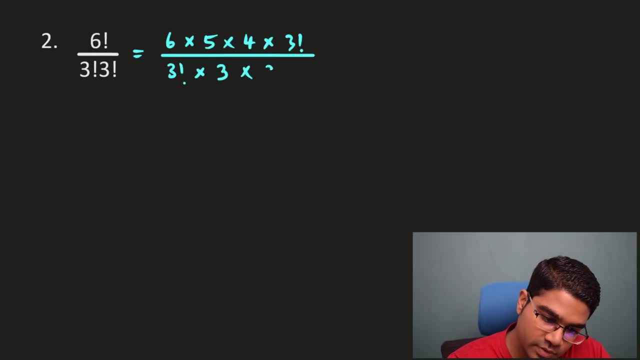 So this will just become times three times two times one, Now three factorial and three factorial. you get one Three factorial divided by three factorial Three times two is of course six, which means this will become one as well. So all that we are left with is five times four, which is twenty. 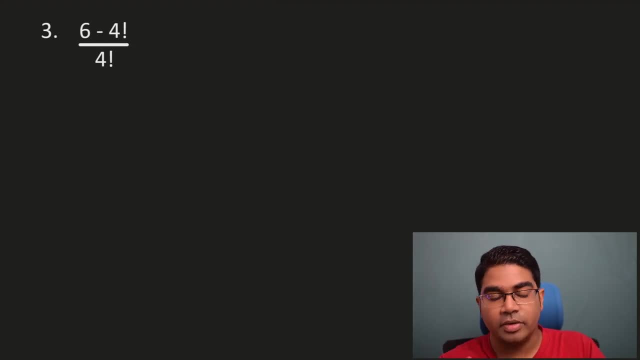 Let's try one more. What if we have six minus four factorial, over four factorial? So we know that six actually has four factorial, because six will be six times five times four factorial. So we can write everything in terms of four factorial. Let's do that first. 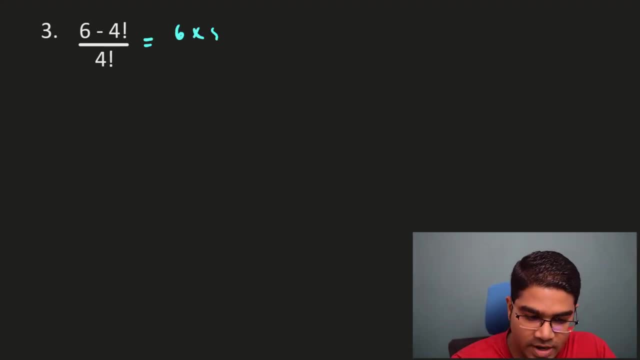 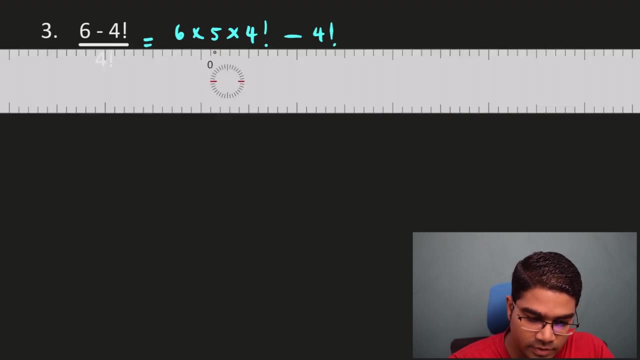 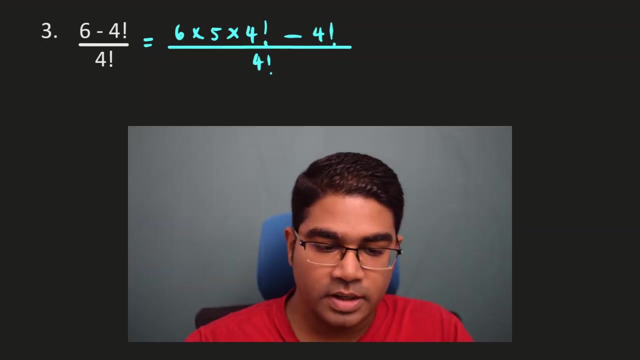 So this will be equals to six times five times four factorial minus four factorial divided by four factorial. So now let's see what happens to this. So there is two ways to do this. First way is you can factorize four factorial and then you can just cancel them out. 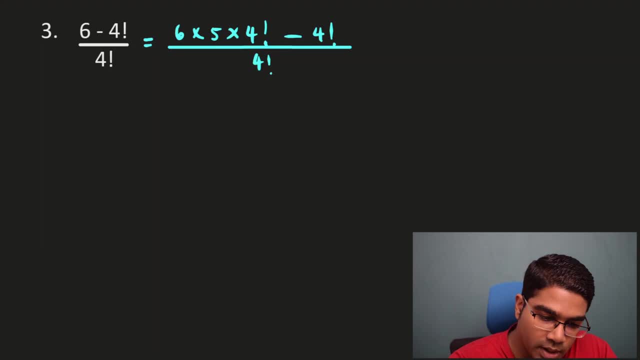 You can eliminate it, because four factorial over four factorial is one, But we can use another way. So six times five is thirty, which means there are thirty four factorials minus one four factorial. Four factorial is one, four factorial over four factorial, So here we actually get thirty minus one. 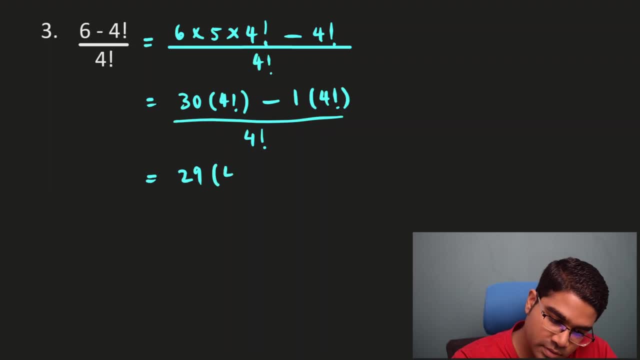 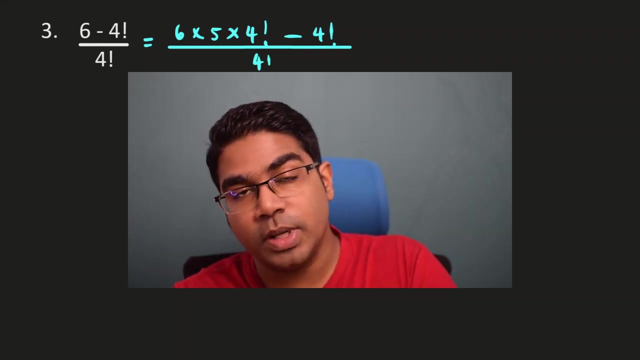 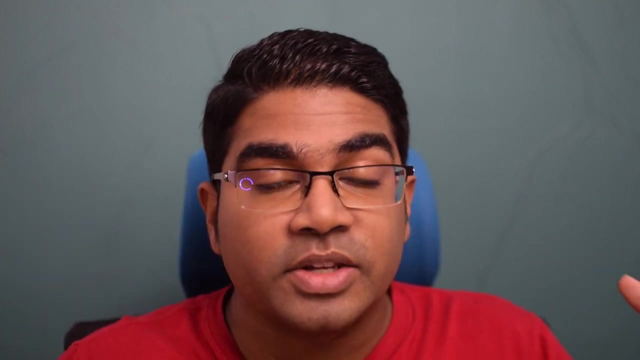 You get twenty nine. four factorials divided by four factorial. So once again, four factorial divided by four factorial, you get one and the answer is twenty nine. So this is another way to do it, if you don't like factorization. Now let's look at permutations, where we actually have more objects to arrange than the number of positions to fill. 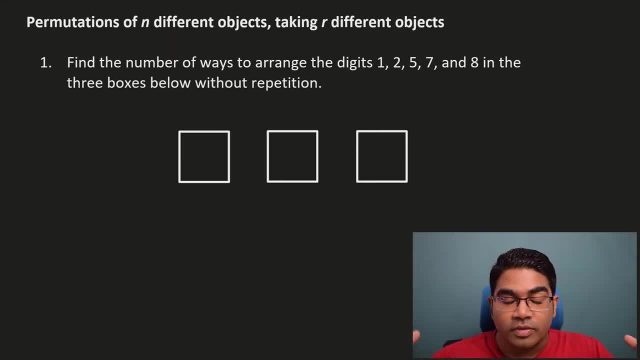 So the number of objects to arrange, The total number of objects to arrange, we normally label as N. N is all the objects we have to put into place, Whereas R is the number of places to fill, The number of positions to fill. So let's look at this question. 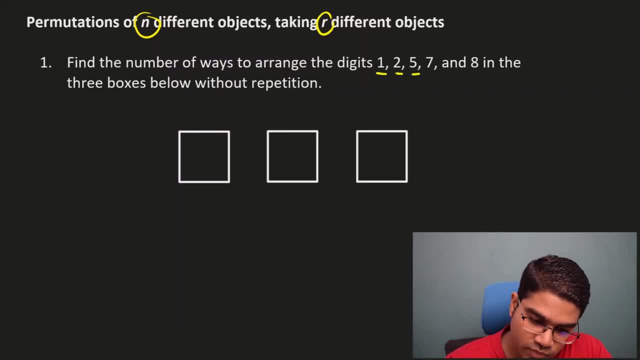 Find the number of ways to arrange the digits one, two, five, seven and eight in the three boxes below, without repetition. So here we have a total of five choices. So this is actually N, N is equal to five, And then we only have three positions to fill. 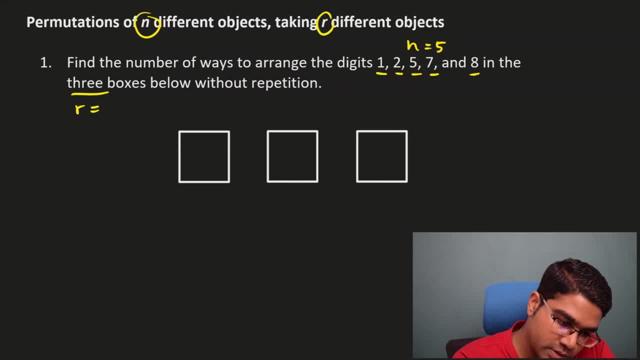 Three places to arrange them. So this is R. R is equal to three. Let's use multiplication rule first. So in the first position we have a total of five choices. We can still put all five numbers, So this will be five. 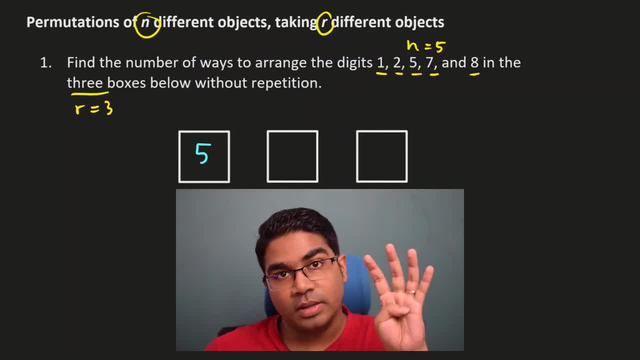 In the second position, since we've already used one. this is without repetition, So we only have four left. So therefore, we fill four for the second position, Because we have four choices. Now the same logic applies: After you've used two, you only have three left. 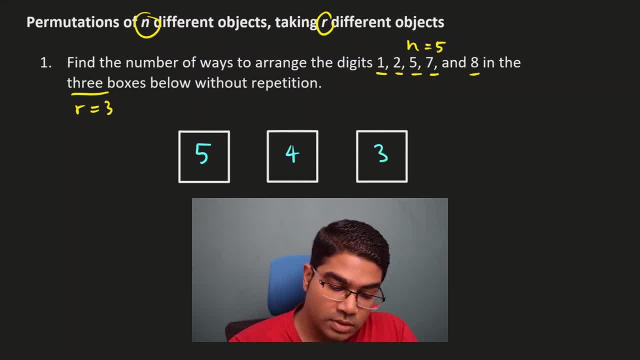 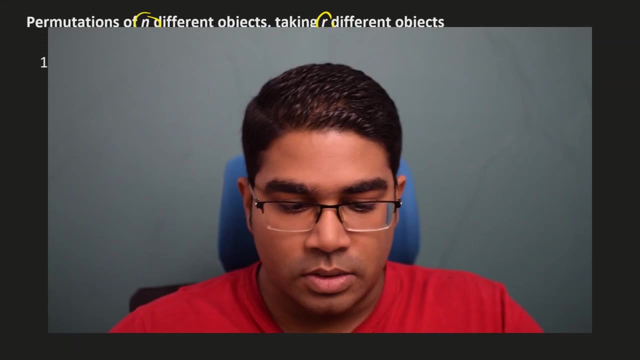 In the third position we have three choices, So the total number of ways we can arrange them will be five times four times three. This is not equal to five factorial, Because five factorial will be five times four times three times two times one. So how do we represent this? 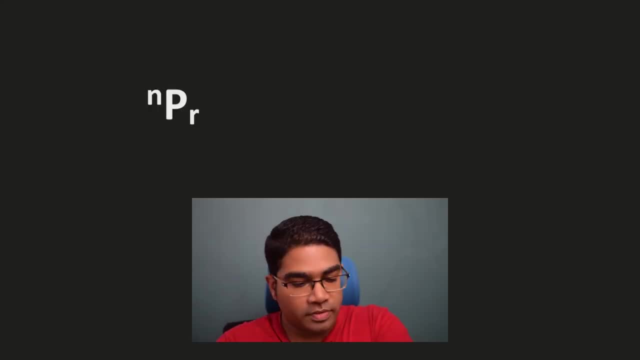 Here we can use the permutation formula. So what's the formula for permutation? It is NPR. Now, sometimes you will see this written as NPR. It's actually the same thing. It doesn't matter whether the N is written as a superscript or a subscript. 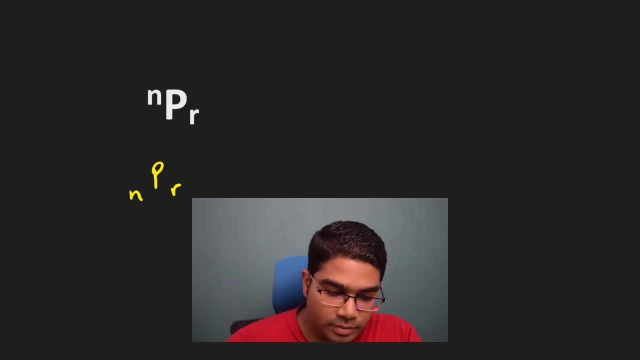 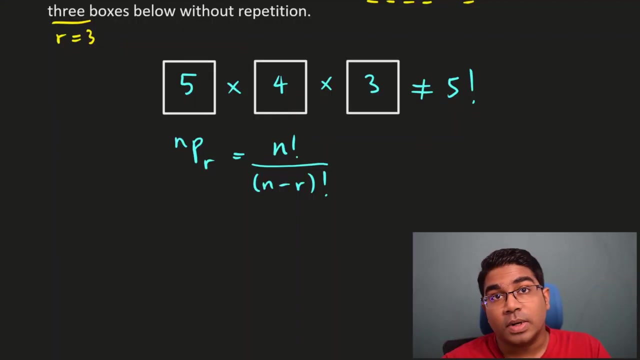 It means the same thing. So what is NPR? NPR is equal to N factorial divided by N minus R factorial. Let's apply it to the question. So what is our N and our R? N was five, R was three, So let's just fill that in. 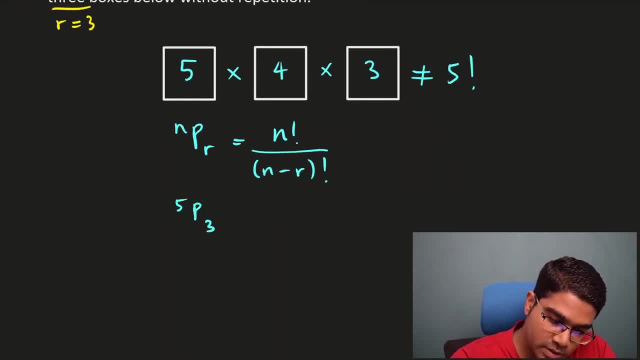 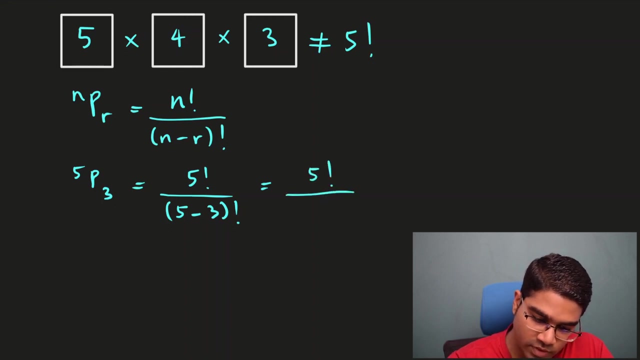 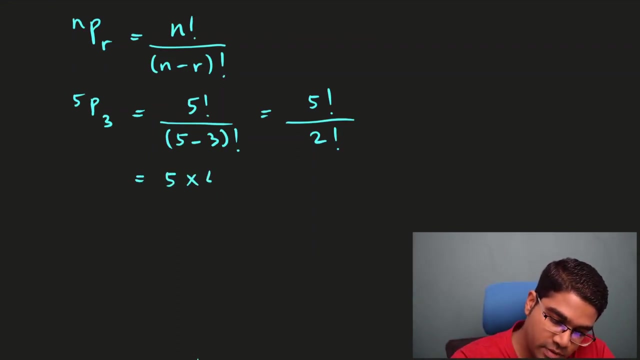 Five P three is equal to five factorial over five minus three factorial. Now this is actually equal to five factorial over two factorial, And this is equal to five times four times three times one, And this is equal to five times four times three times two factorial divided by two factorial. 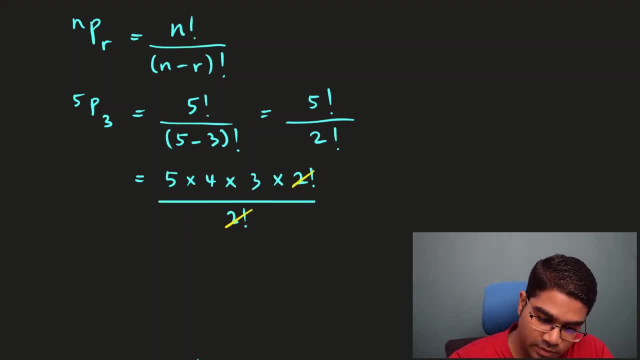 And we can eliminate two factorial, because two factorial divided by two factorial is just one and one. What we end up with is five times four times three. In the end, we have ended up with exactly what we did using the multiplication rule: Five times four times three. 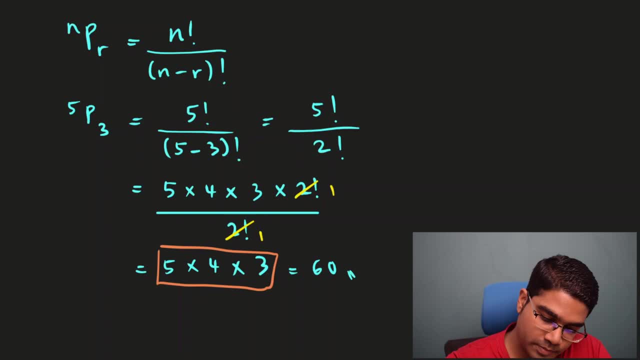 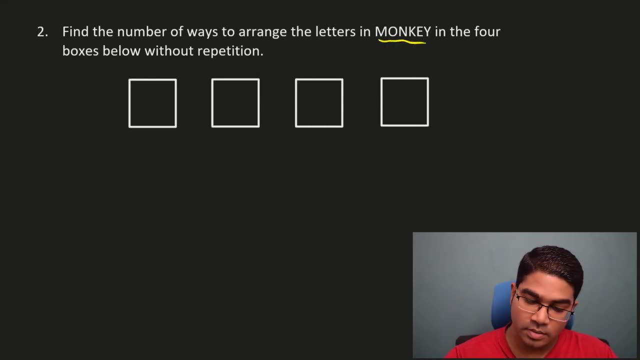 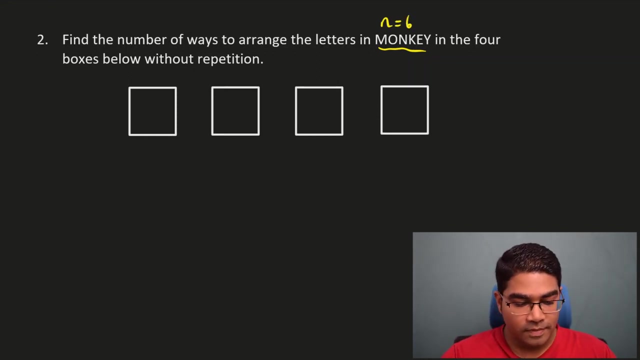 And the answer here is sixty. Let's look at another example. Find the number of ways to arrange the letters in monkey. Here we have a total of six letters, So N is equal to six. This is all our choices in the four boxes below. 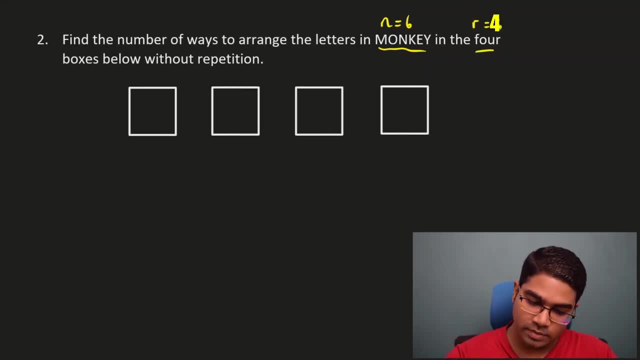 Four is R, without repetition. Let's use multiplication rule and then we will use the formula According to multiplication rule. in the first position we have all our choices, So we have a total of six letters, So six choices here. In the second, we have used one. 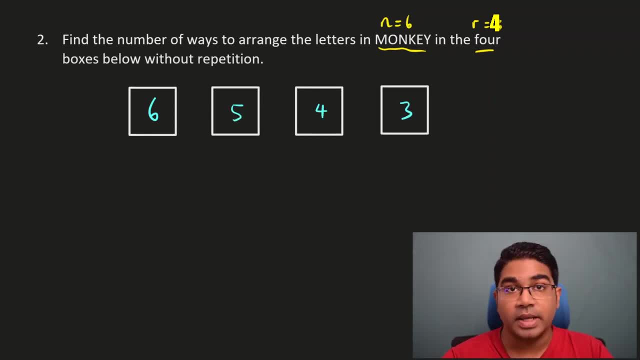 So five remaining and then four remaining and then three remaining. So by multiplication rule the number of ways will be six times five times four times three. Let's use the formula. So by formula we will have N. P. R. N is six. 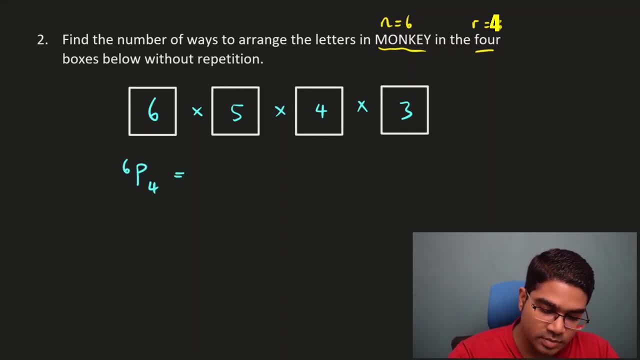 P R is four. Six P four. This will be equal to six factorial Over six minus four factorial. This is equal to six factorial over two factorial. Now we can do the working. You can just keep your calculator. So this will be six times five times four times three times two factorial divided by two factorial. 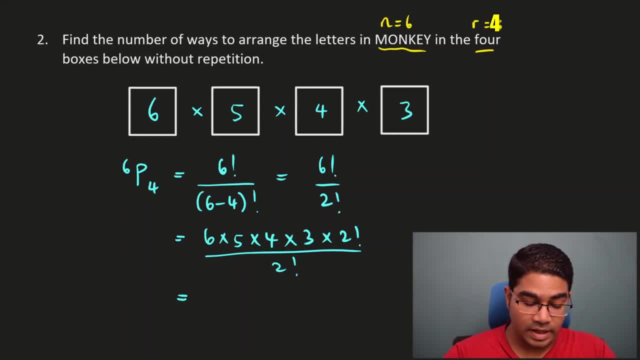 And so the answer we get is three hundred and sixty. You can try and see. You will get the answer. You will get the same thing here as shown Six times, five times, four times three. So it doesn't matter which way you use. 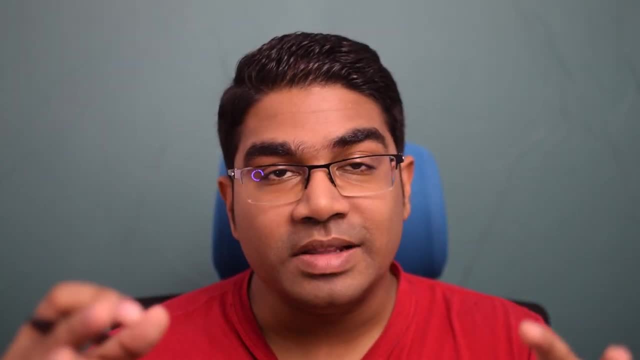 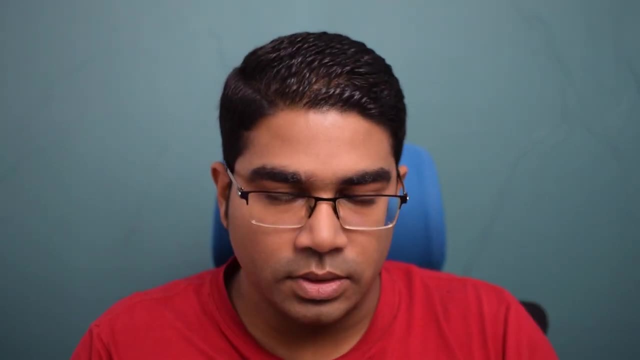 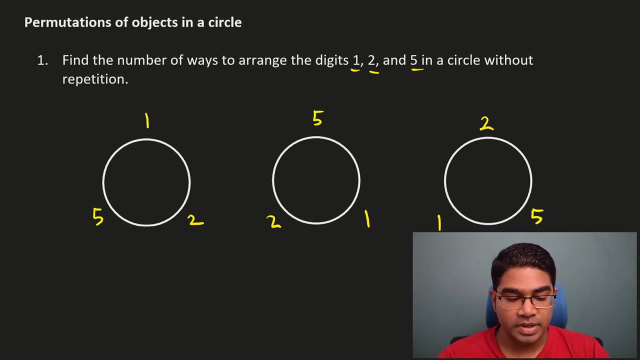 Total number of ways is three hundred and sixty. So far we have been arranging things in line, So we are always forming a line. Now what if we form a circle? Let's look at the example here. Find the number of ways to arrange the digits one, two and five in a circle without repetition. 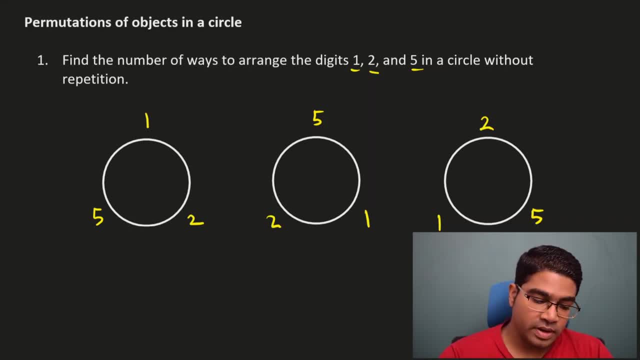 Let's look at these three arrangements. here You can see we have one, two, five and then five, one, two and then two, five, one. if this were a straight line: One, two, five, five, one, two and two, five, one. 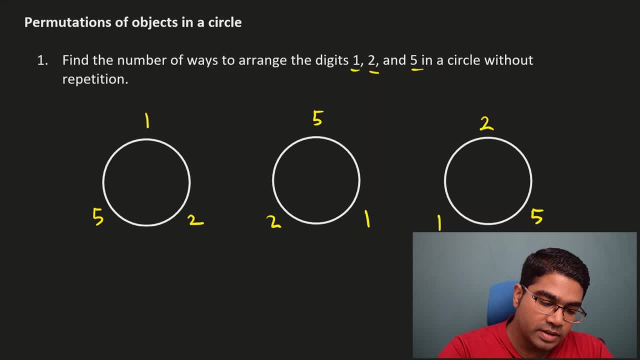 are three different arrangements, But since they are in a circle, you can see all we are doing is rotating the circle. It is actually the same arrangement. We are just turning the circle. It depends on where you look from. So these are considered to be the same arrangement. 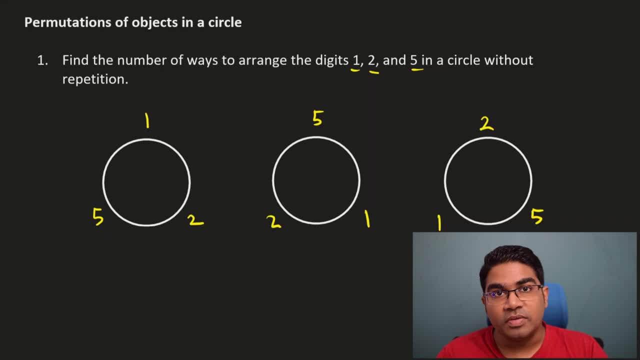 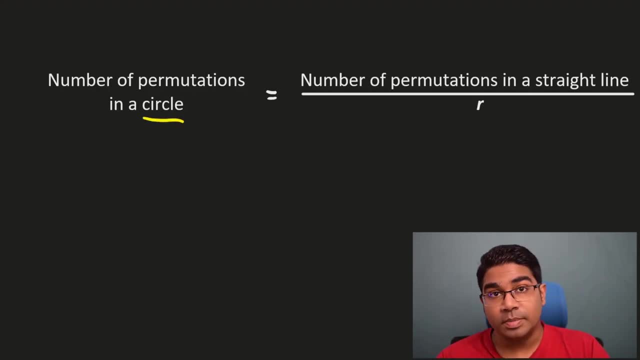 What happened here is that the total number of arrangements has been reduced three times. This is the logic that we are going to use. The number of permutations in a circle would simply be the number of permutations that you get in a straight line, but since they form a circle, 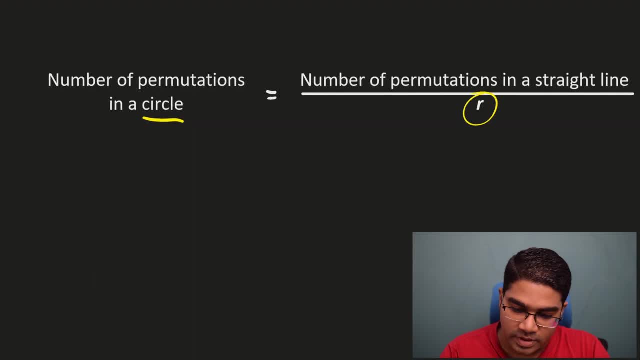 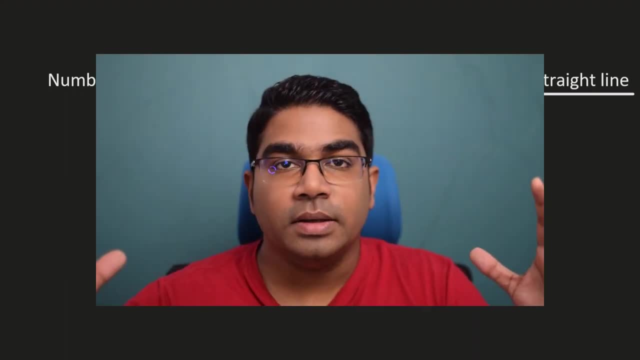 it is reduced by r times. So we divide by r. What is r? Remember, r is the number of positions to fill. So, whatever you would get in a straight line, do as usual: Find the number of ways, the number of arrangements, and then you divide by r. 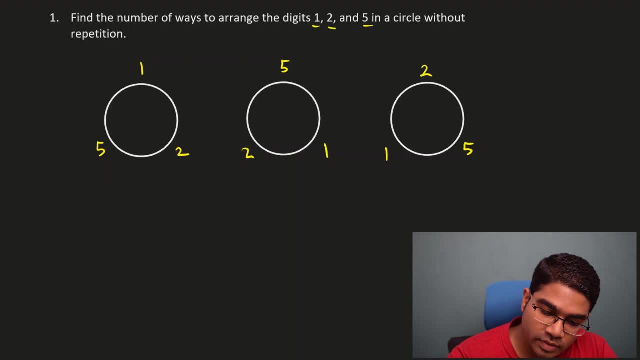 That's all. Let's apply it to this question. We have three to arrange, So n is equal to three And we have three positions to fill, So r is also equal to three. There is something very interesting when n is equal to r. 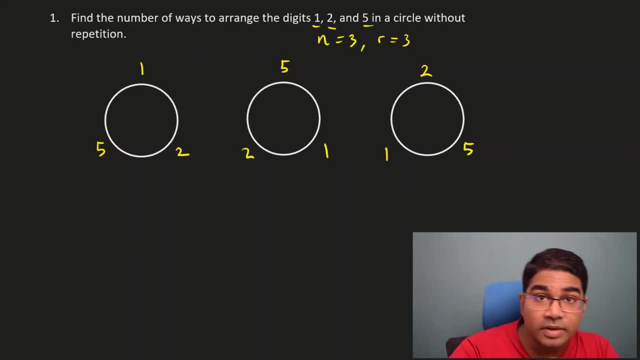 So let's apply the formula. This would be if it were a straight line first. If it were a straight line, we would have 3p3.. And this is equal to three factorial over three minus three. Three minus three factorial is zero factorial. 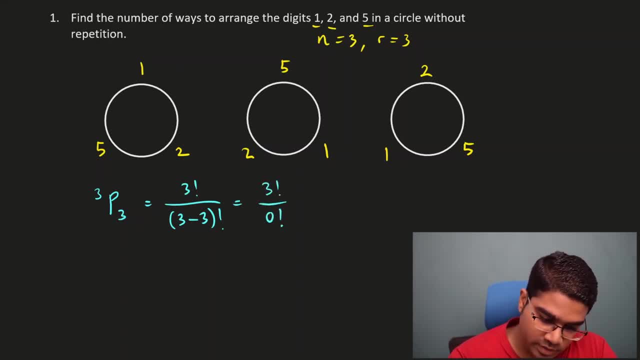 So we have three factorial over zero factorial. By definition, zero factorial is one. So we have three factorial over one, which is just three times two times one which is six. So here I want to focus on the fact that when we have npn. 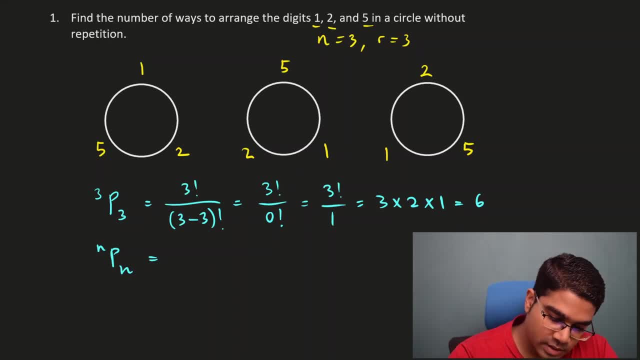 this is the same as n factorial. as you can see here, 3p3 is equal to three factorial. Now this is if it were a straight line, So the number of ways when it is in a circle would be equal to. we take the number of arrangements. 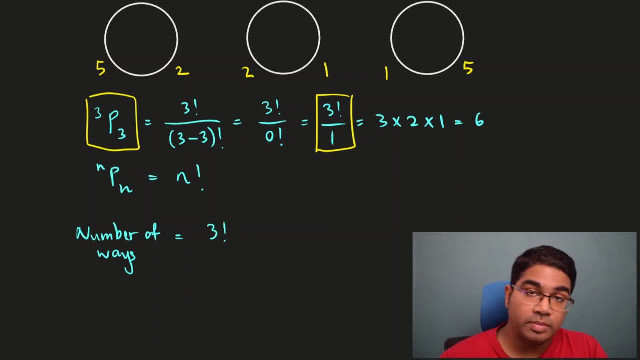 if it were a straight line, which would just be three factorial, because this is 3p3.. And then you divide by the number of positions that we can fill, which is also three. So divide it by three, This will lead to three times two times one over three. 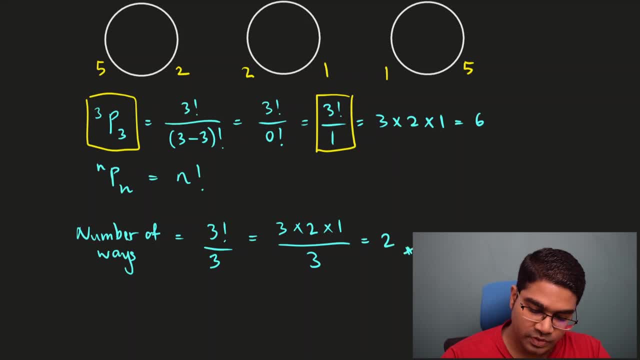 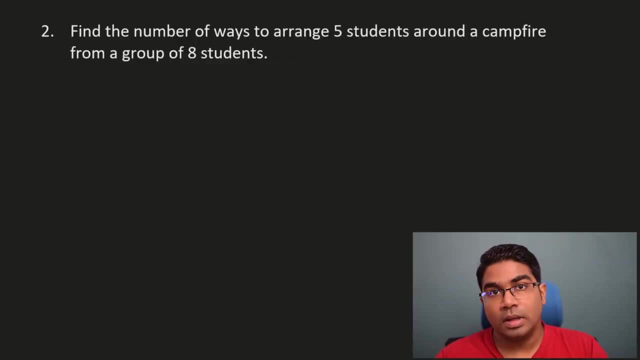 which is just two. So there's only two ways to arrange the three letters in a circle. What if n is not equal to r? Let's look at this: Find the number of ways to arrange five students around a campfire from a group of eight students. 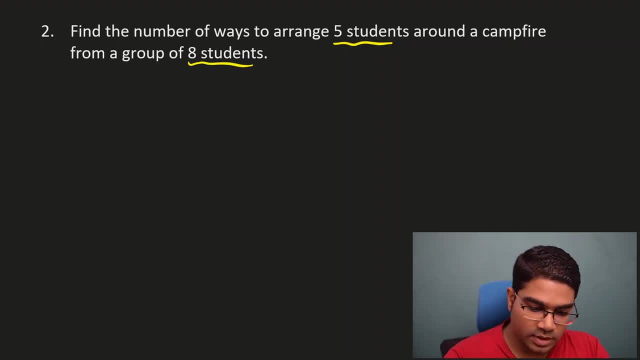 So there are eight students, but we are only picking five. So here n is equal to eight and r is equal to five. How do we do this? We use the same concept, So the number of ways will be equal to what we would do. 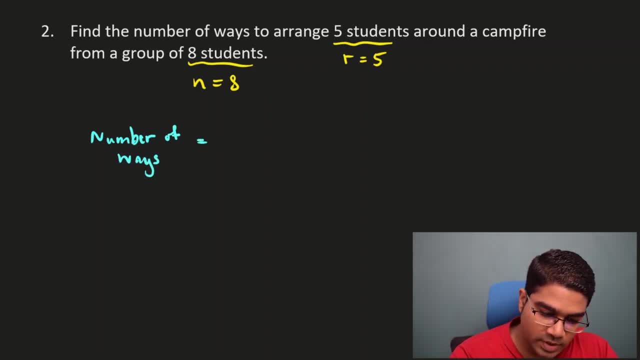 if they were arranged in a straight line, divided by r, So number of ways is equal to npr. eight p five. This is what we would do if it was a straight line, And then you just divide by r, So r is five. 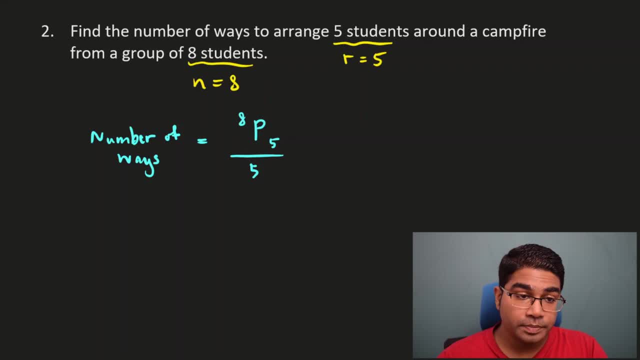 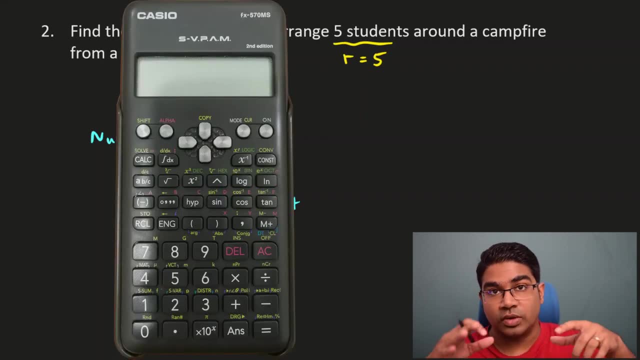 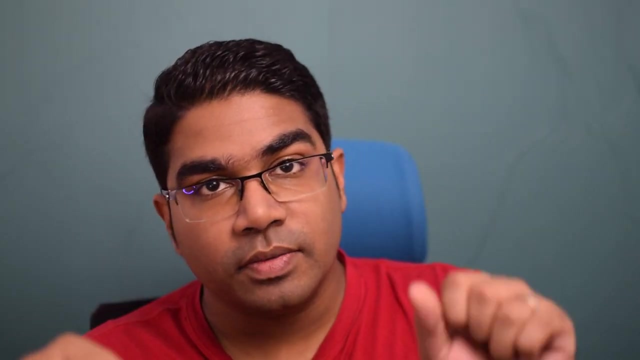 So divided by five. Key this into the calculator and you will get one, three, four, four. How do we use a calculator to do permutation? As you can see the calculator on the screen, look for this. You will see npr. If you were trying to do eight, p, five. 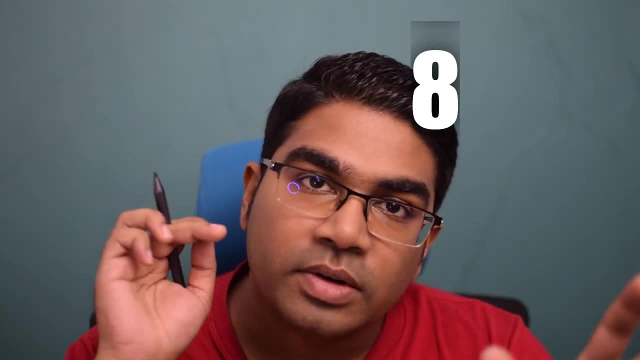 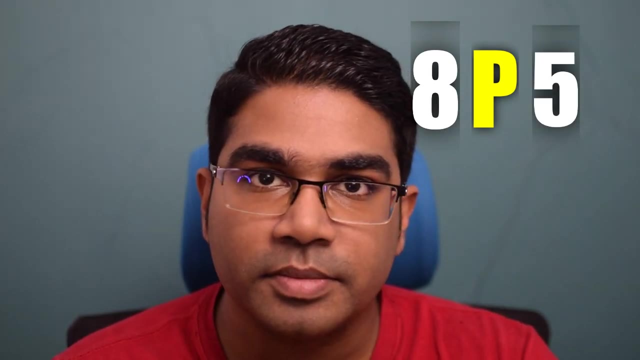 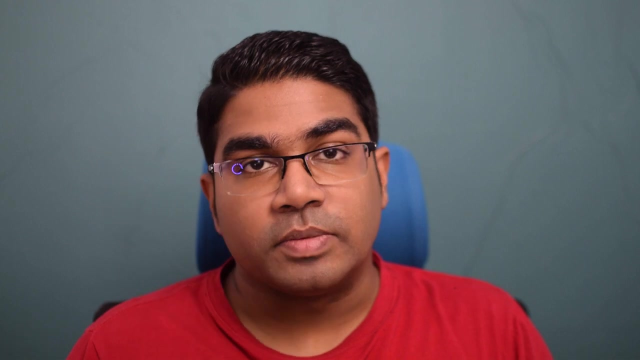 you press eight first, and then you press shift and that button to get the p, and then you type the number five. That's how you do it. So far we've been dealing with unique objects, So every single object is different. What about if we want to arrange? 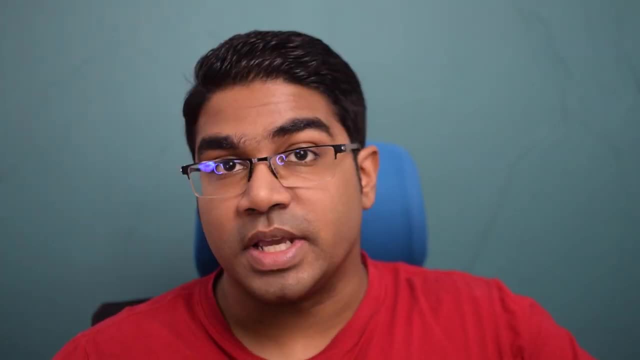 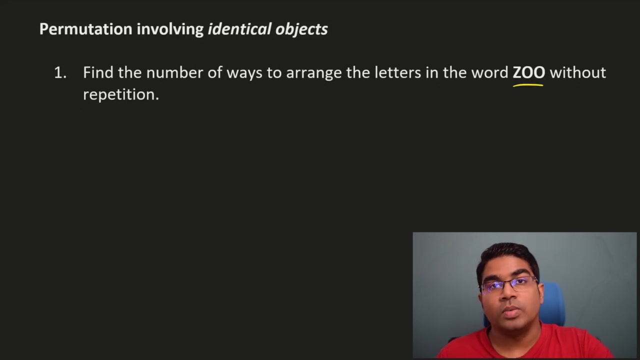 objects. where we have identical objects, Find the number of ways to arrange the letters in the word zoo without repetition. So when we look at zoo we have z o o. O is repeated. How do we deal with this If we count them as different? 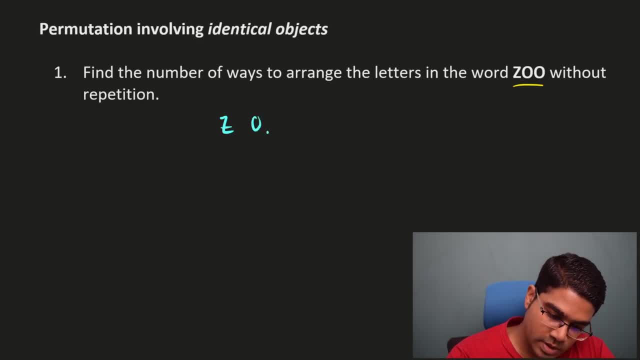 let's label them as z o one and o two. If they were different, then z o one o two and the arrangement z o two o one would be considered different arrangements. But they are the same. They are identical. O and o are identical. 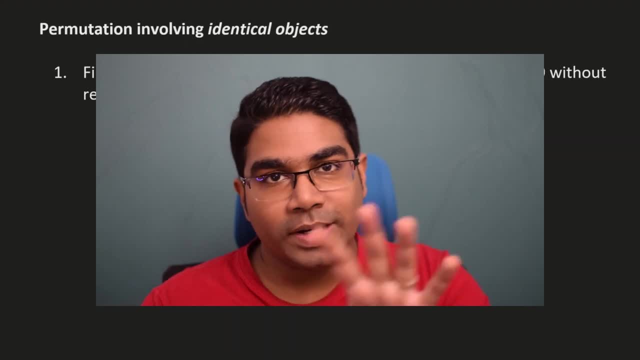 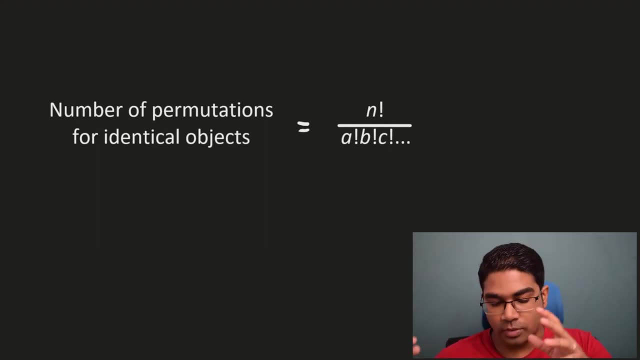 So these two arrangements are actually the same. When it comes to this situation, we use the formula n- factorial over a factorial times b factorial times c- factorial, and so on. So what does this mean? n is the same as before, The total number of objects. 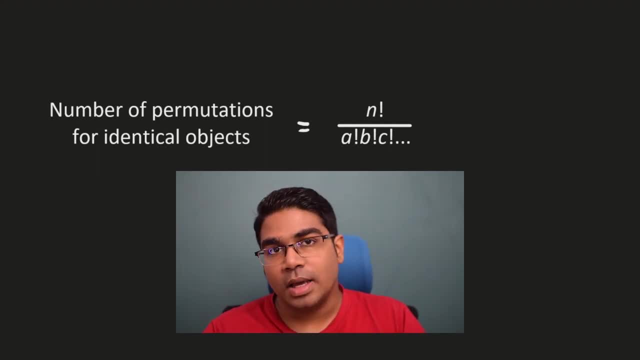 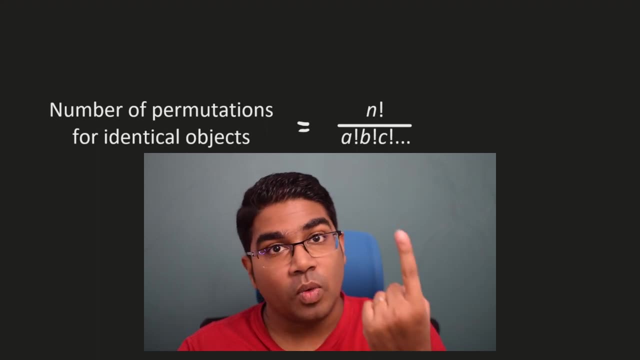 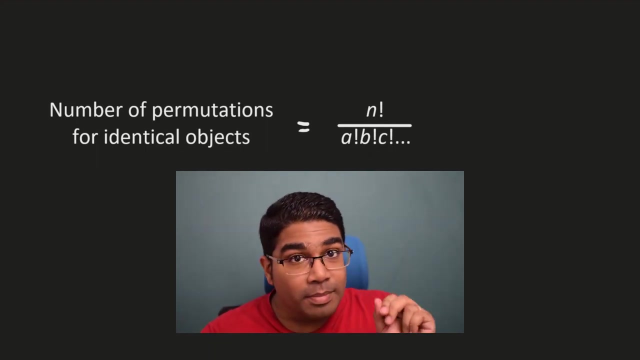 we have to arrange. a, b and c are the number of identical objects for each object. In our case, we only have one object that has identical objects present, So we have o. a value will be the number of identical objects, So the number of o's. 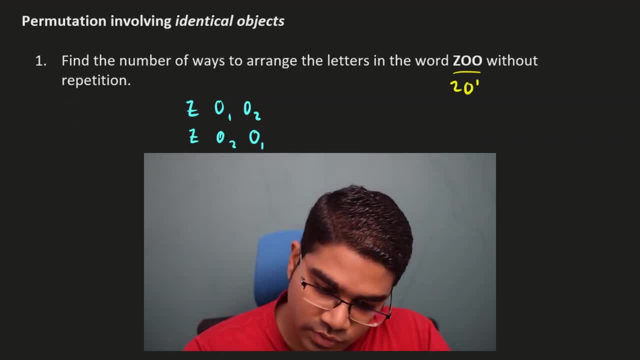 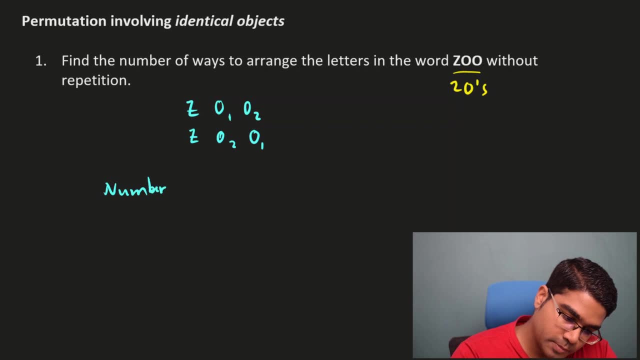 In the word zoo. we have two o's, So let's apply the formula. Number of ways will be equals to n factorial n is three. We have three letters, So three factorial over. since we have an identical case, we have two o's. 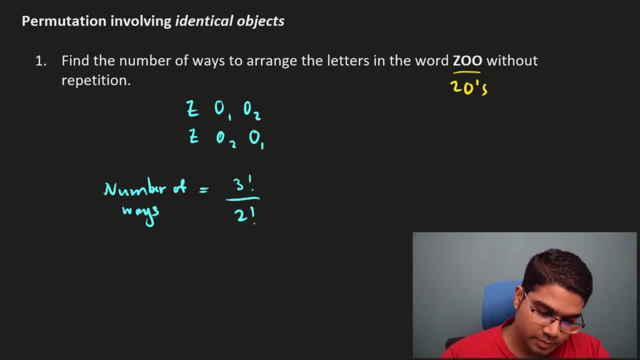 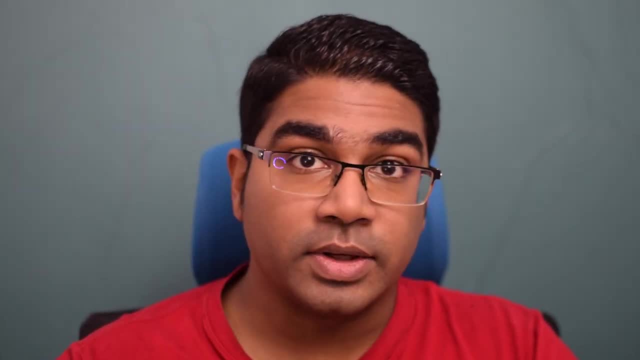 So this will be two factorial, This will simply be three. What if we have more than one identical object? Let's look at the next question: Find the number of ways to arrange the letters in the word coconut. So in the word coconut we have: 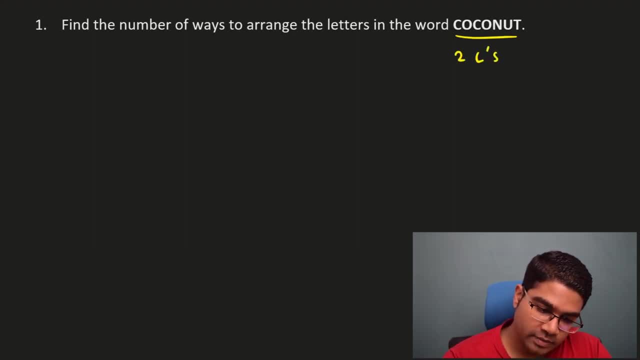 two c's and we have two o's, So now we have two identical objects. How do we deal with this? Let's apply the formula. Number of ways is equals to n factorial. There are a total of seven letters here in coconut. 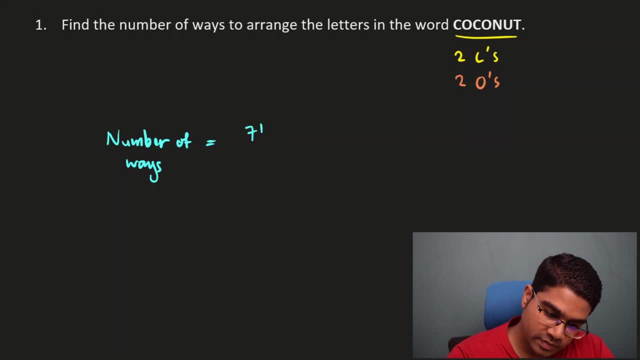 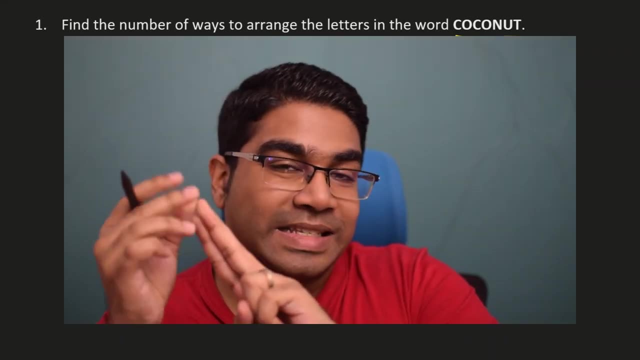 So n is equals to seven, Seven factorial divided. by Now we have two identical objects. We look at the number of identical objects In each for each object. So for o we have two and for c we have two. So we do them separately. 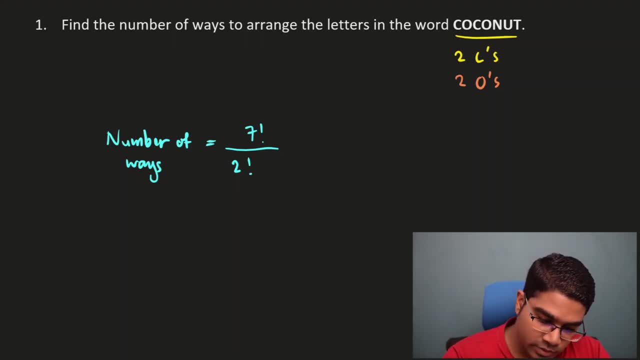 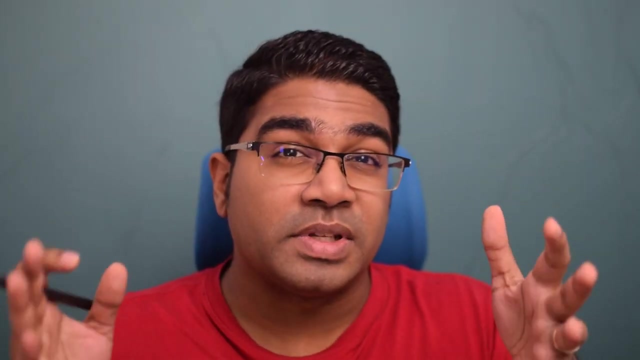 So it will be two factorial- This is for c, and then two factorial for o. Just key this into your calculator and you will get one thousand two hundred and sixty. This is how we deal with multiple identical objects. Certain arrangements have specific conditions that you need to meet. 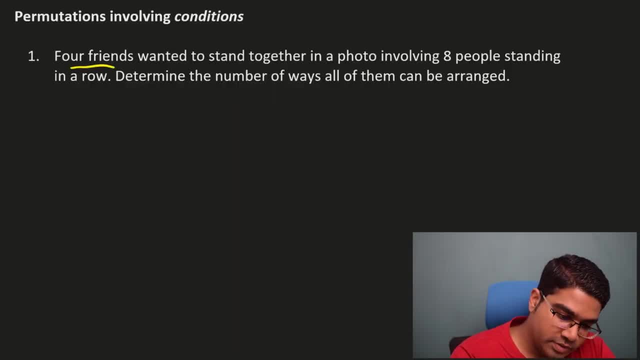 Let's look at those questions. Four friends want to stand together in a photo involving eight people standing in a row Determine the number of ways all of them can be arranged. Now we have eight people, but out of the eight people, four want to stand together. 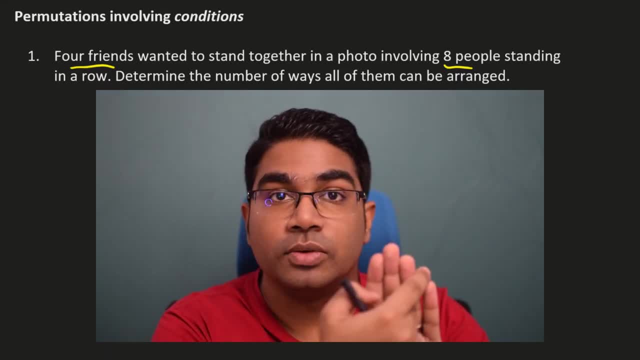 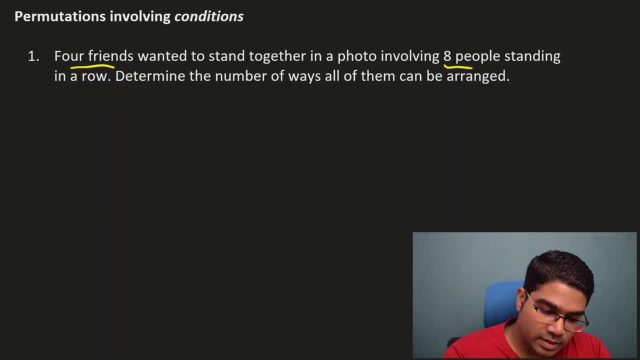 Among the four. it doesn't matter who stands besides who, but all the four of them want to be together. In this case we involve some grouping here. Let's write them as individuals first. So we have eight people. that would be X, Z. 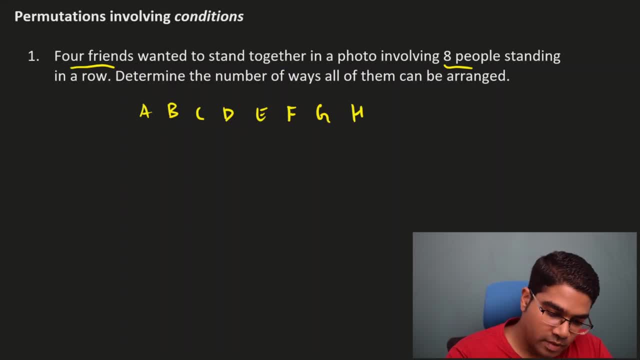 D, E, F, G and H, Eight people. Out of the eight people, four must be together, So we group them first. The first step is to group them. So let's call this X. So when we group it as X, 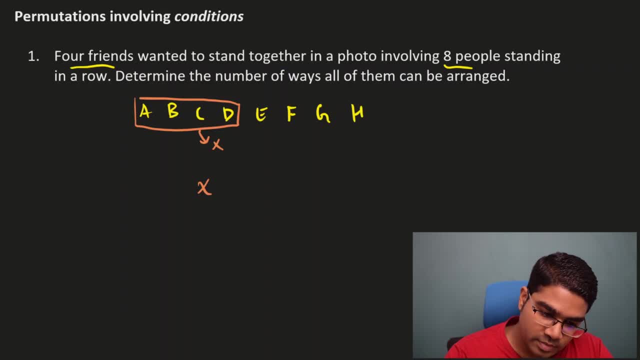 then we only have five to arrange, five objects. That would be X, E, F, G and H. So X will always be together. This is how we do it. The first step is grouping. First we find the number of permutations. 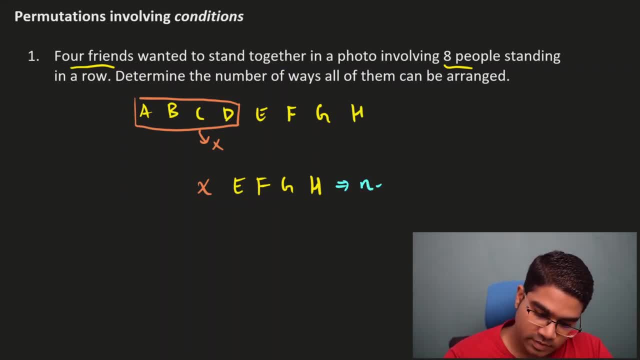 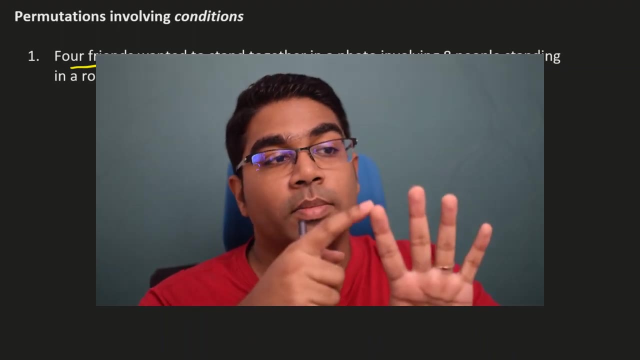 with the five Here: N is five, R is five. So this is just five factorial. The number of ways here is five factorial. This is not including the number of different ways. The four of them can arrange within X, So within X itself. 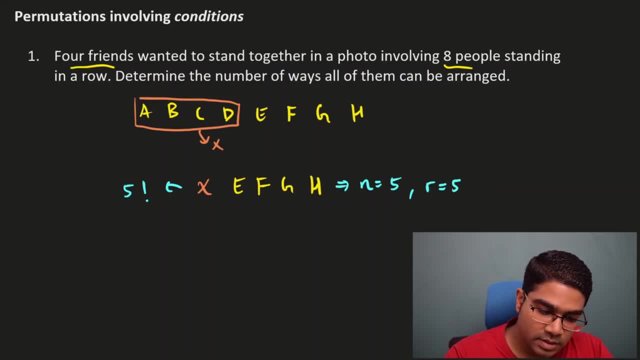 we have different arrangements. What do we have within X? Within X, we will have four factorial, because N is four, R is four, So we have four factorial arrangements within X itself. Now how do we combine these together When we have this situation where we have 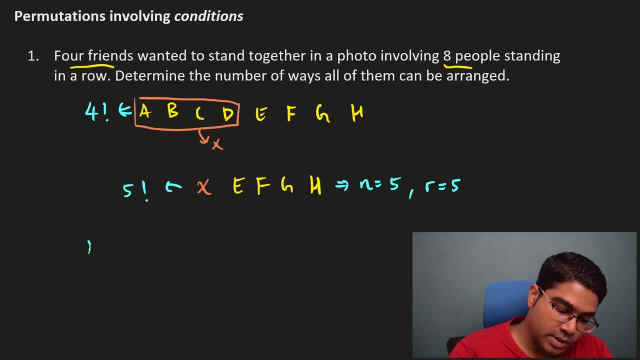 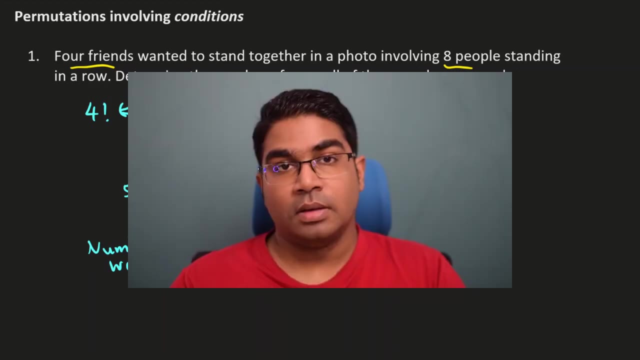 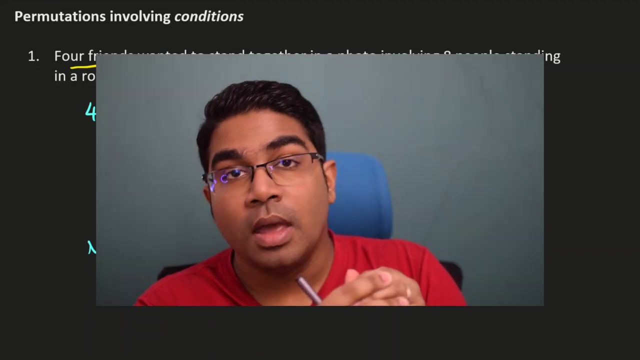 grouping. so we do multiplication. The total number of ways would be five factorial times four factorial. Using the calculator we would get two, eight, eight, zero ways. So in any kind of situation where you need objects to be side by side, we group them first and treat. 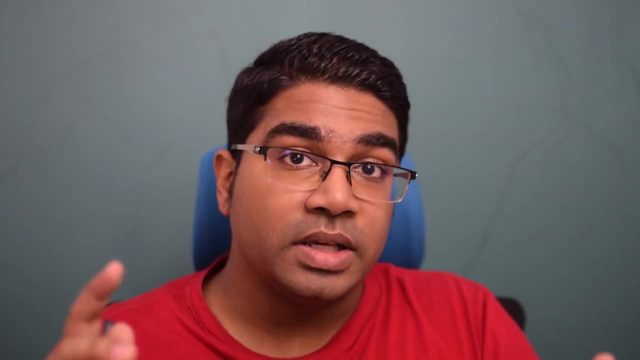 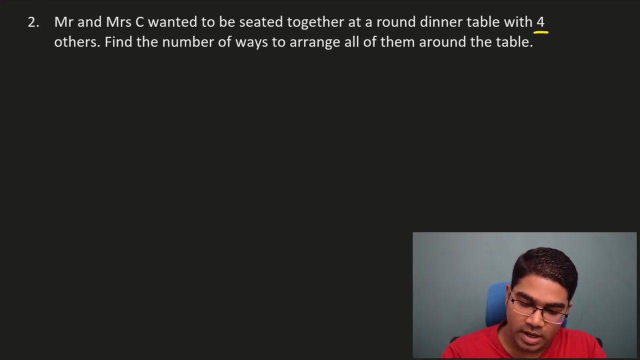 them as a single object. Now let's try another question, but this time, what if it is in a circle? Mr and Mrs C wanted to be seated together at a round dinner table with four others, So they want to sit together with four others, which means 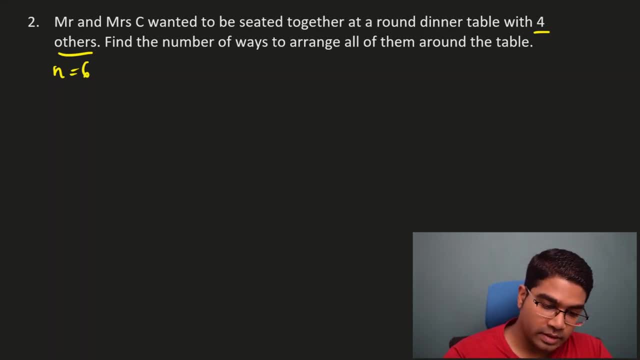 N is equals to six. We have a total of six objects to arrange. Find the number of ways to arrange all of them around the table. Now let's look at a straight arrangement, which is A and B and F, But two of them want to sit. 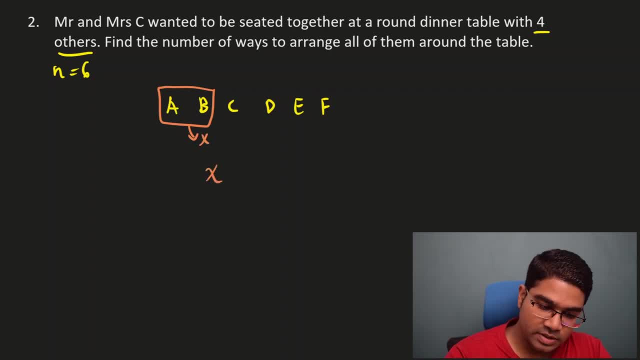 together. so we need to group them: A and B. let's call it X, So we simplify this to X, C, D, E and F. So now we only have five to arrange, Five to arrange in five positions. So the total number of ways: 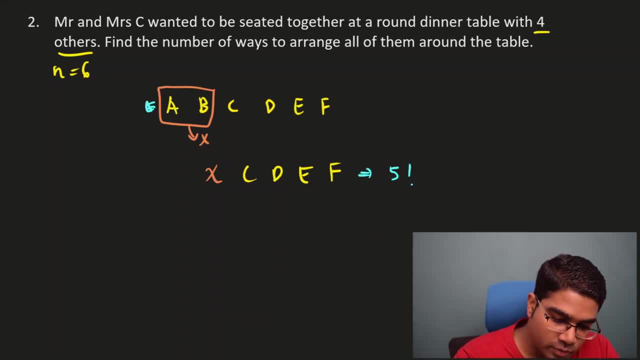 they can be arranged within the group itself will be two factorial, because we have two arranged in two positions, So two P two, two factorial, Just like we did earlier. the number of ways here will simply be five factorial times two factorial. However, we must remember that 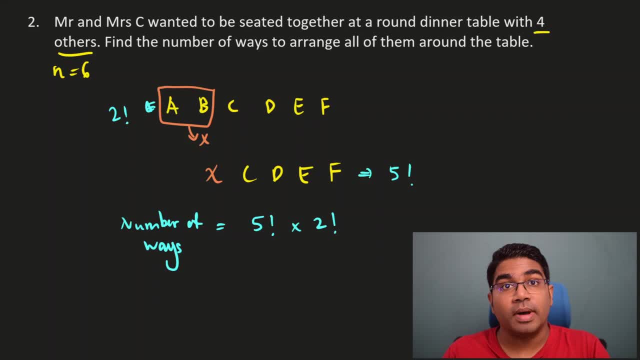 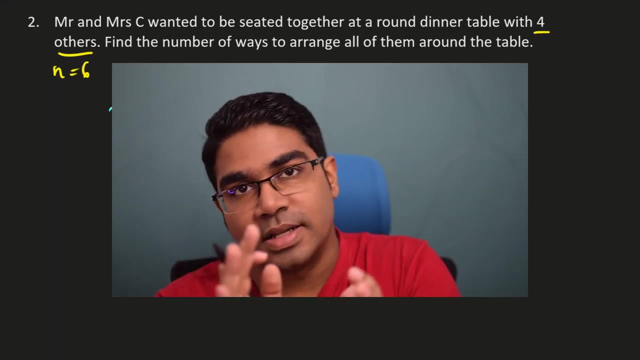 this is an arrangement in a circle. If you arrange in a circle, then you arrange in a straight line, And then we have to divide by R. So what is R here? Which R do we use? Do we use five or six? Just remember. 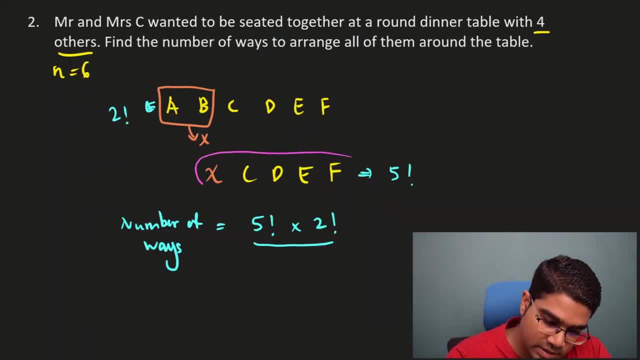 which you arrange in a circle. So we actually arranged five in a circle. We were arranging this in a circle. We didn't arrange A, B, C, D in a circle. Now let's look at the other condition, Find the number of ways to. 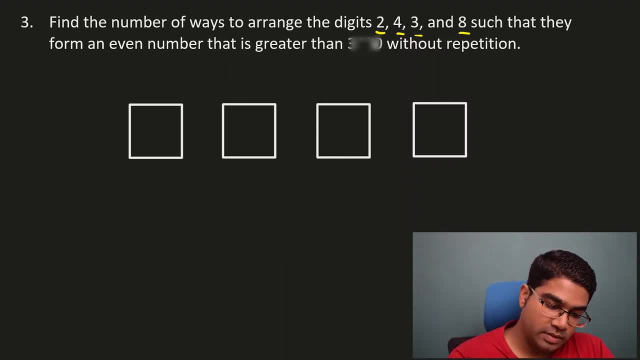 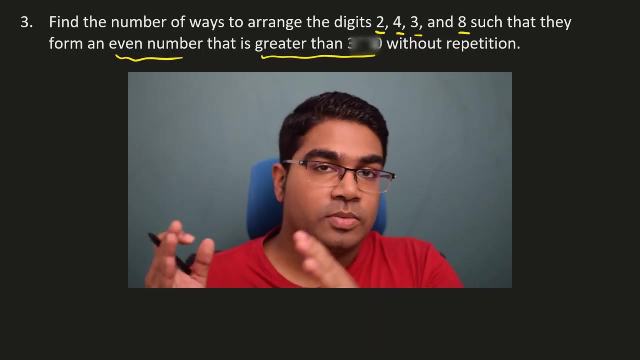 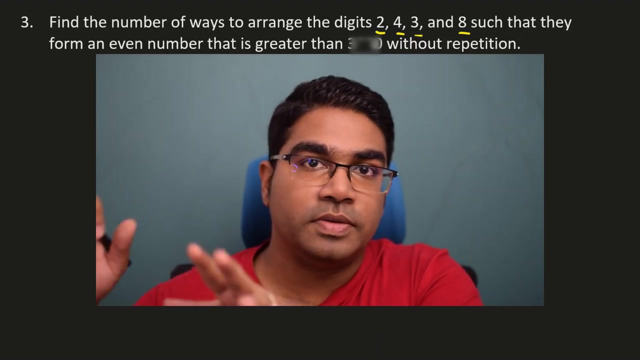 arrange the digits two, four, three and eight such that they form an even number that is greater than 3000, without repetition. Here we have conditions like this. It is best to draw out the boxes to fill in the position. The first condition is: 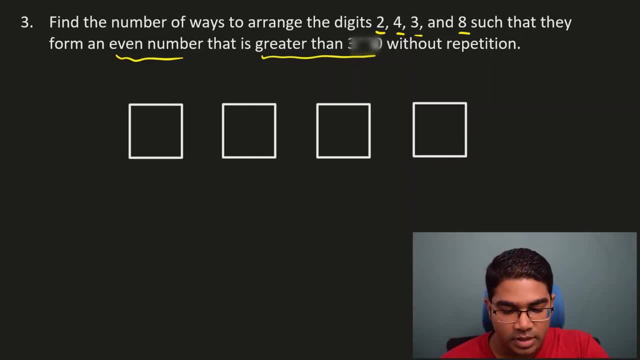 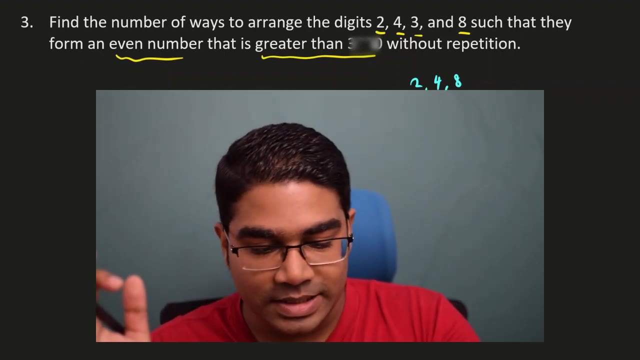 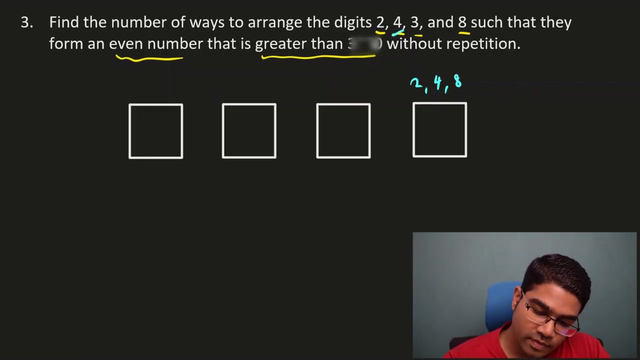 that it has to be an even number. For the whole number to be an even number, of course, only the last digit has to be an even number. So what we can place in the last position would be a number greater than 3000. If it. 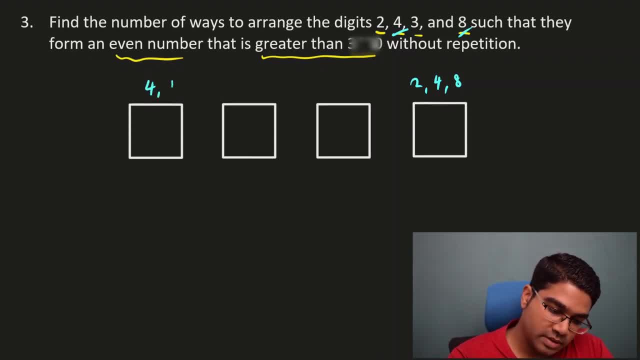 has to be greater than 3000, then we can only choose four and eight. So there are only two possibilities for the first position Now we have the conditions met, but you have to remember this is without a number. you need to split it into two. 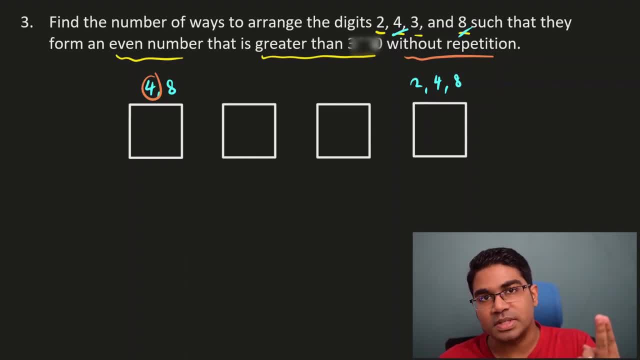 combined events, One involving four at the first position and another one involving eight at the first position. Let's go with choosing four first. So if we chose four, then there is only one option here, Only four. We don't put anything in the 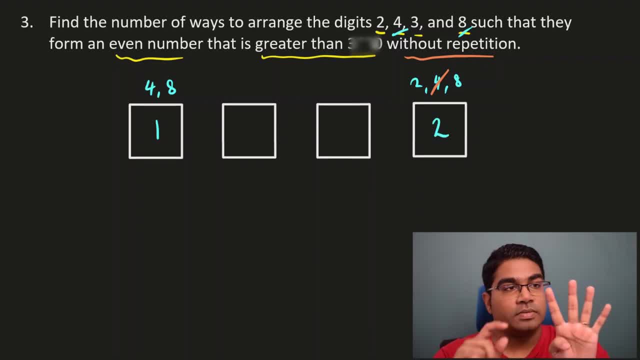 second position. So we have a total of four digits. We have already filled the first position with one digit, the second position with another digit, So all we are left with is two digits. So the number of choices we have for the second position is: 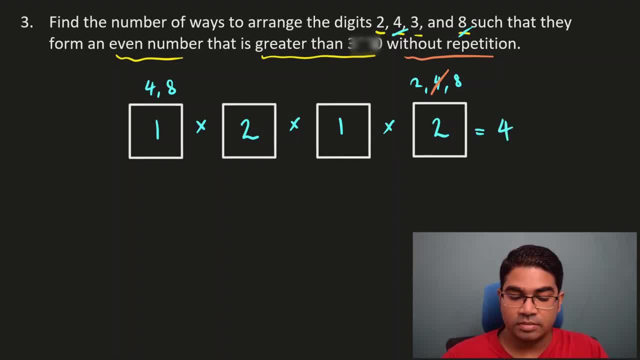 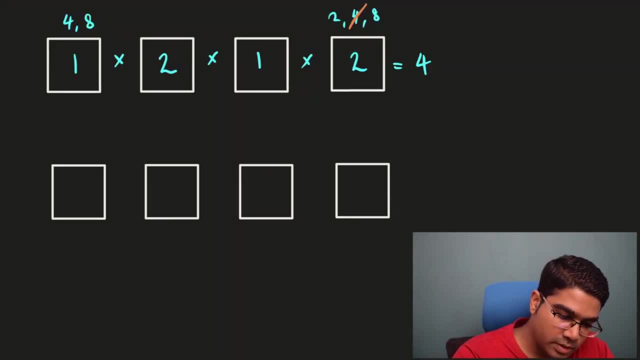 actually two. There is a total of four ways. Now we also have the option of having eight at the front. So let's do that Again. let's write our options. So now we are only using eight, and then we have a choice of. 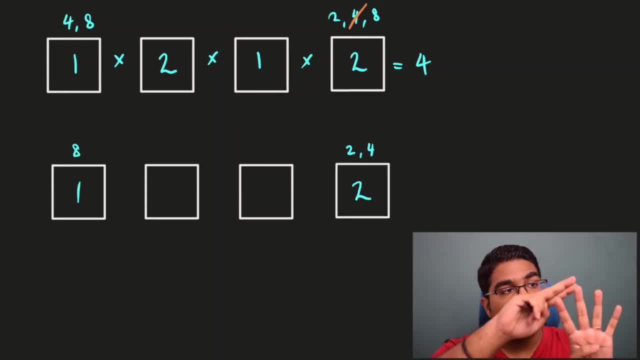 two and four at the end, because we cannot use eight anymore. So we have one choice for one. So we multiply all together Again. here also, we have four different ways of arranging with eight at the front. Now how do we find the total number? 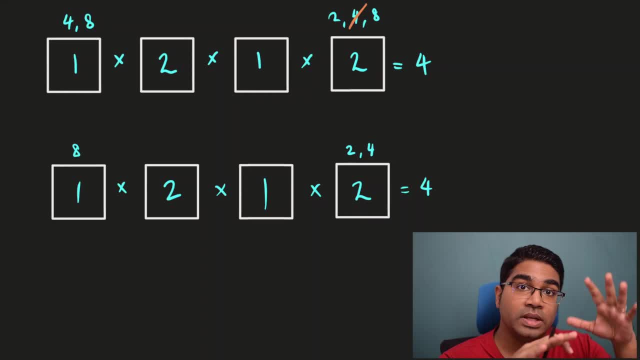 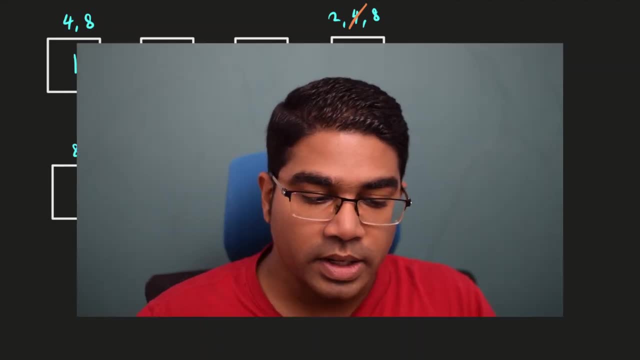 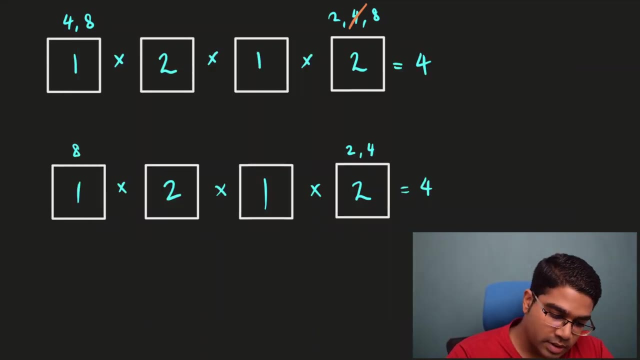 of ways. So these are two separate combined events. They are not the same combined event as we did earlier with the grouping, With the grouping. they are not the same. So in this case the total number of ways where you separated them will be equals. 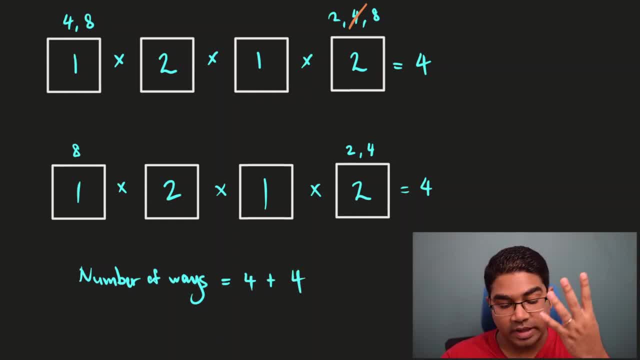 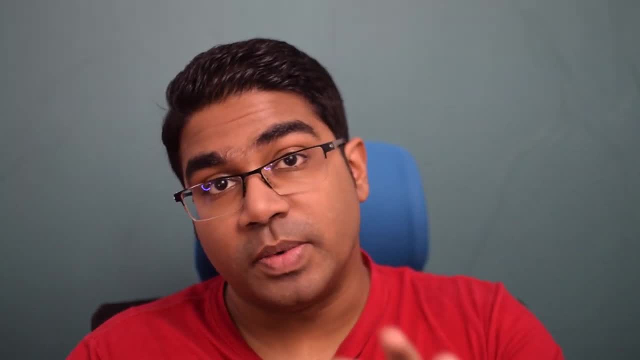 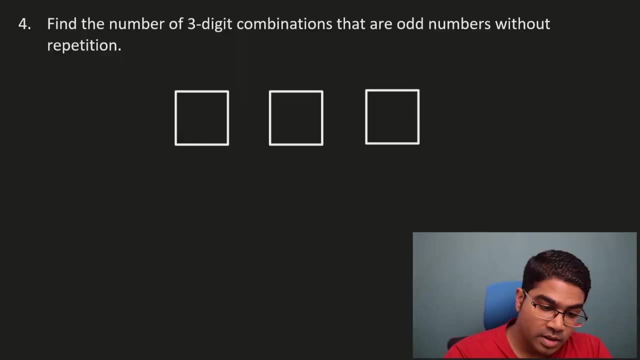 to four plus four at both ways. The first way is four, the second way is four, so this will be eight, Eight ways in total. What if we formed an arrangement with conditions that are odd numbers without repetition? In this case we can use: